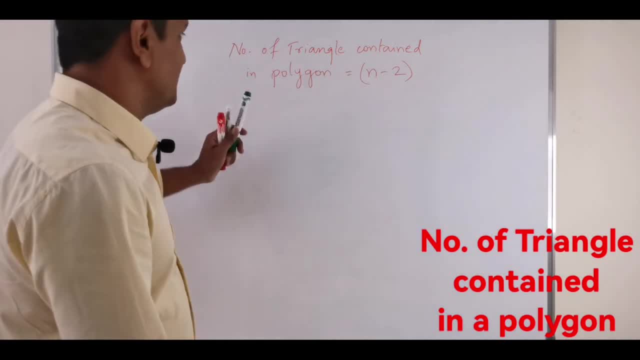 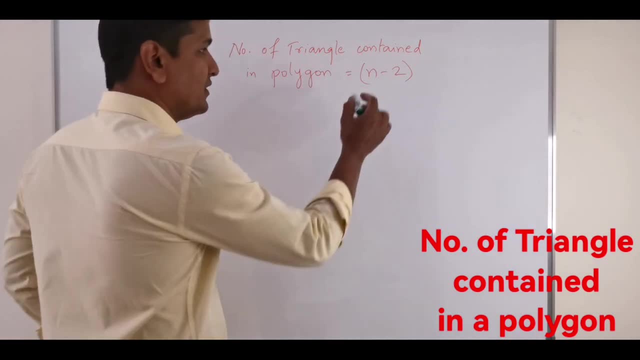 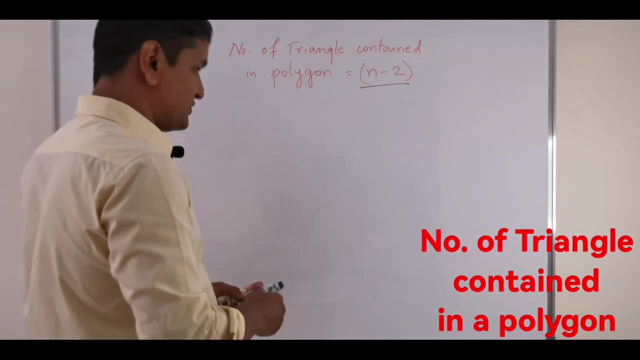 Hi, hello everyone. Welcome to Edwidge channel. Today we will do how many triangles contain in one polygon, How we will come to know. So there is a one formula: n minus 2.. Okay, what is n? n is number of the sides, Suppose I will give you the question like quadrilateral. I want to find 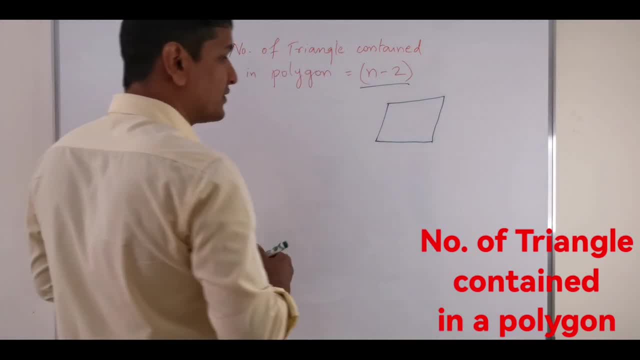 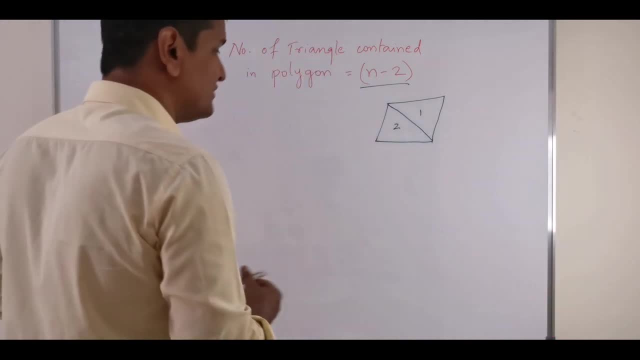 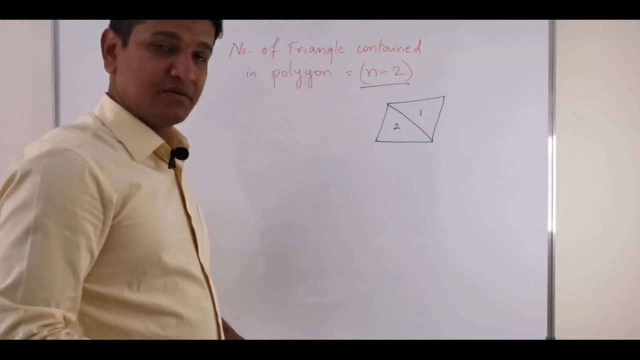 how many triangle in this? So there are two triangles, right, It is very easy. One, this one, this, Okay, how it came by the using the formula For this diagram? it is very easy, But if there is a very big like pentagon or something, hexagon, then it is very difficult to find a. 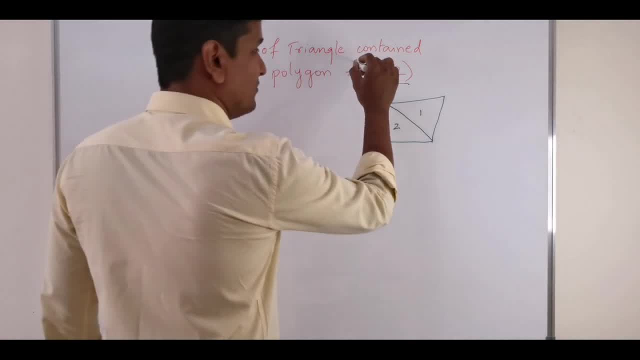 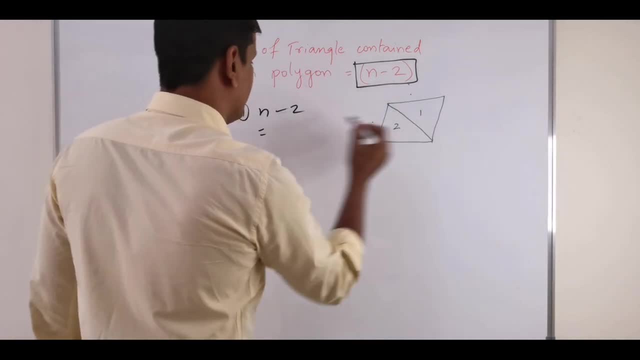 triangle. It is easy, but in a short way we can use by this formula like n minus 2.. So n minus 2, suppose. if I use for this. So how many side for this? 1, 2, 3, 4.. So 4 minus 2, which is 2.. So 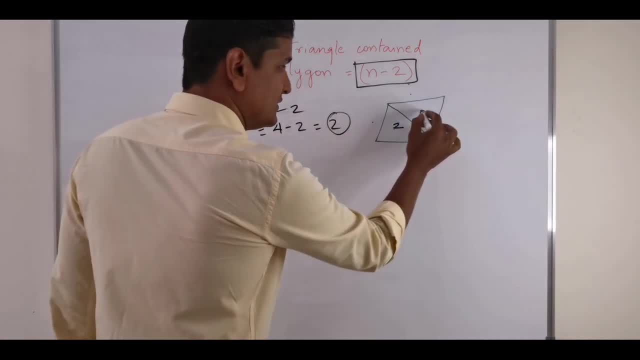 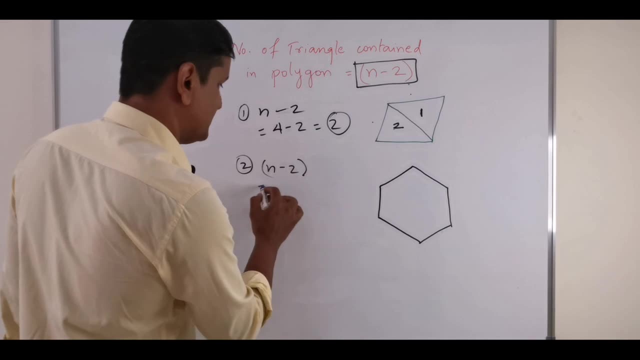 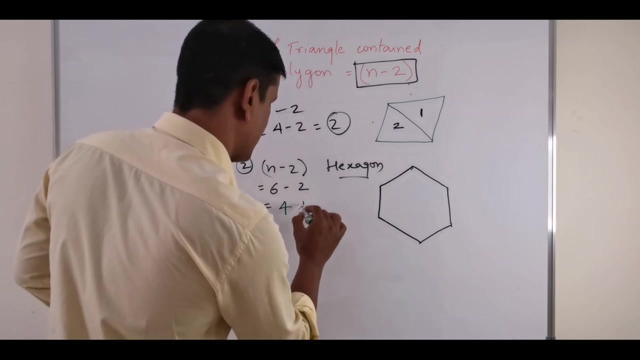 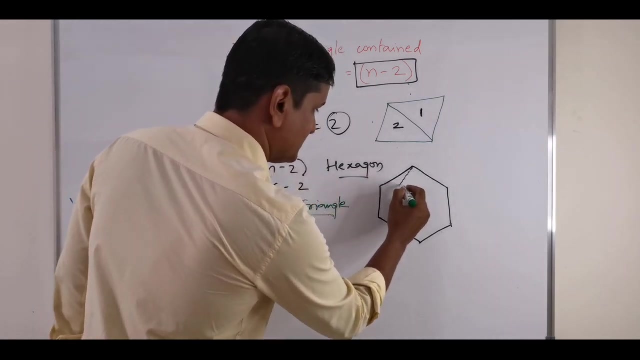 that is why you are able to make two triangle, only One, this and one this. Okay, suppose this is hexagon, right? So hexagon is how many sides? It is 6 minus 2.. So 6 and minus 2 will be 4.. So 4 triangles will be made in hexagon, Okay, so let us see how much So. 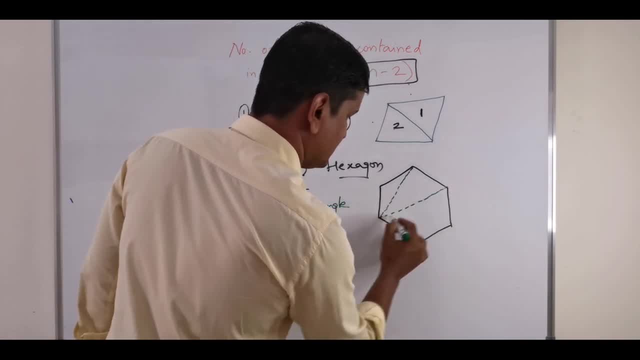 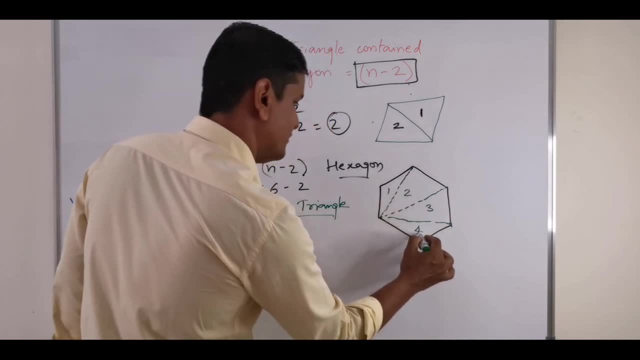 this is 1, this is 2, this is 3 and this one is 4.. So 1, second triangle, third triangle, fourth triangle, So there are 4 triangles. It is made in the hexagon triangle, So this is the way. 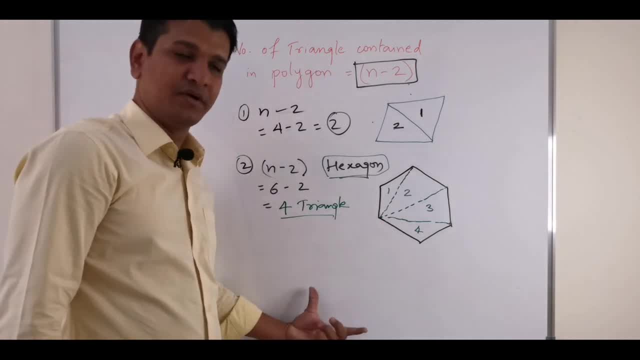 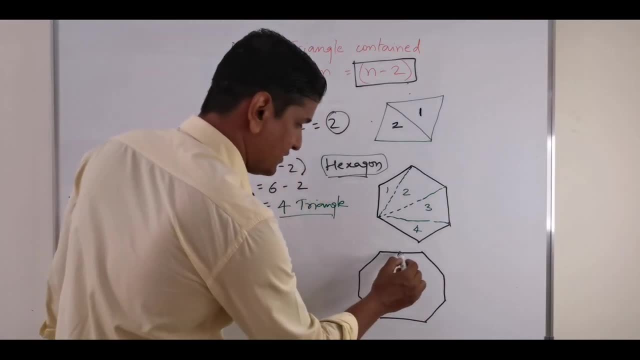 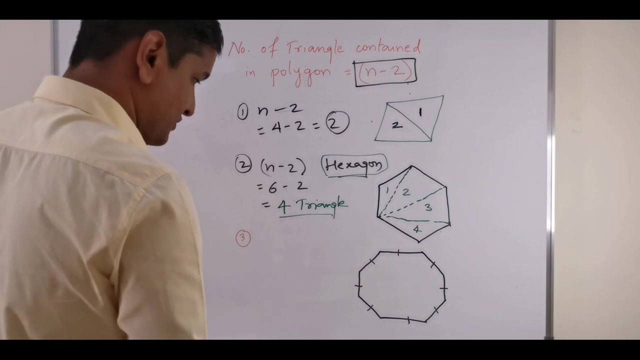 you can find the number of triangle, how much it is contained in one polygon. Okay, use this formula: n minus 2 and you can find this one: How many sides in this? This is called octagon because there are how many sides: 1, 2, 3, 4, 5, 6, 7, 8.. 8 side is there. So in 8 side we can find how.